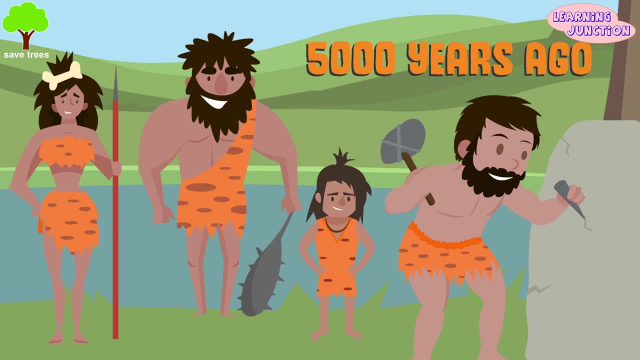 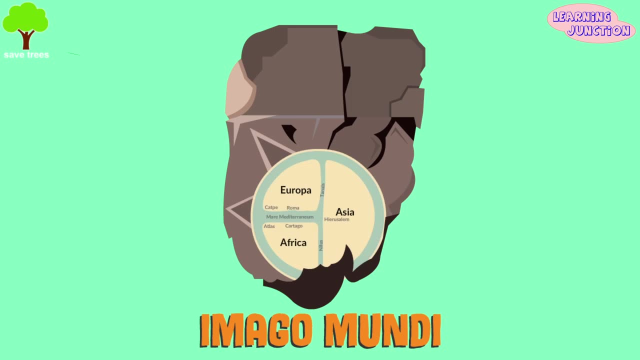 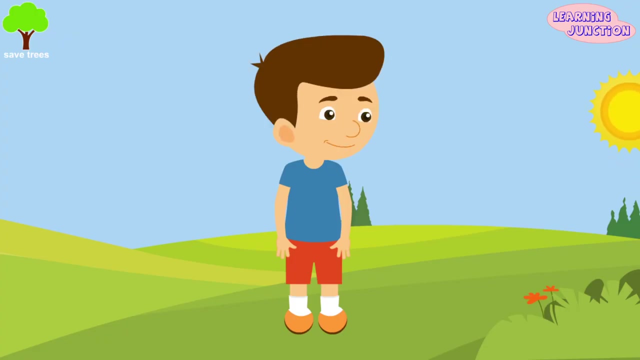 of mapping can be traced to approximately 5,000 years ago. Guys, this is the Imago Mandi. it is considered the oldest surviving world map. It was found in a town called Sephara in Iraq. The sun rises in the east. Stretch out your arms. Your left hand is now pointing east. 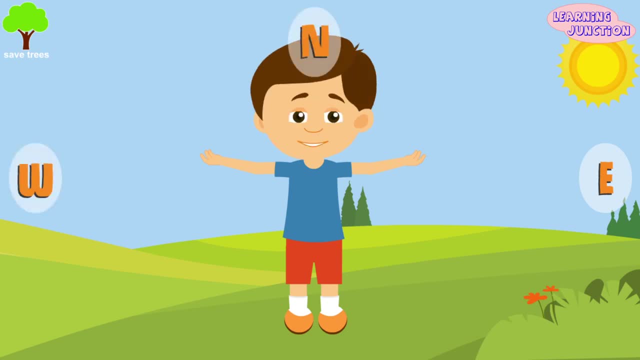 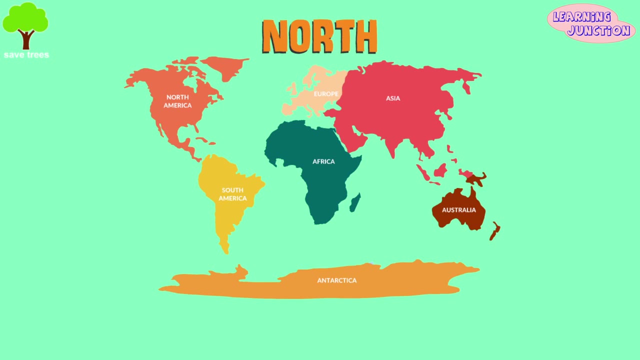 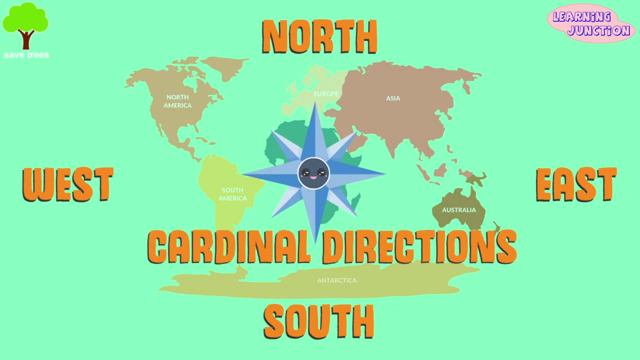 Right hand is pointing west. North is at the top and south towards the bottom. This is the map of the world. North is at the top, south at the bottom. This is east and this part is facing west. These are called the cardinal directions. You can easily see which. 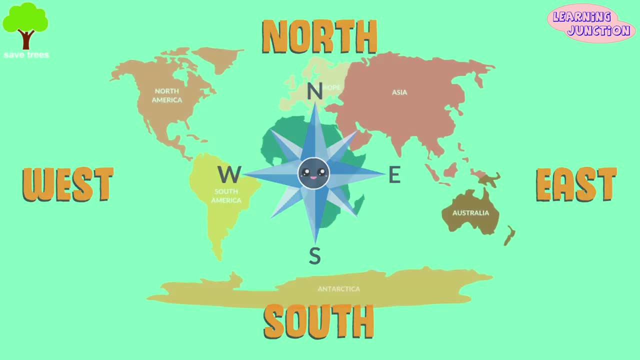 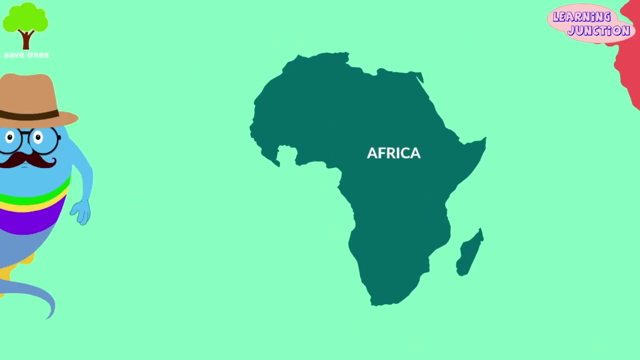 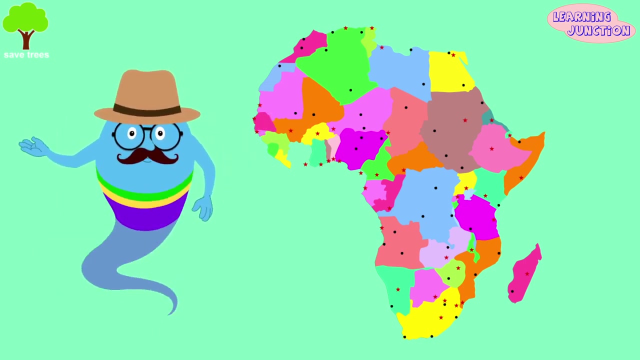 country or continent is in which direction. Different places are shown with different colors so we can easily locate a particular continent. Usually, countries are shown by dots and capitals with a star. There are many types of maps. Let's see the five main types one by one. 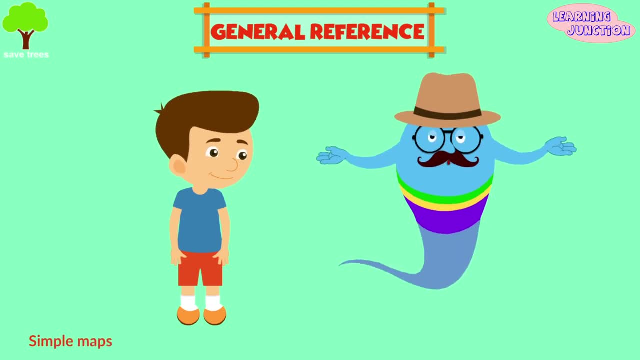 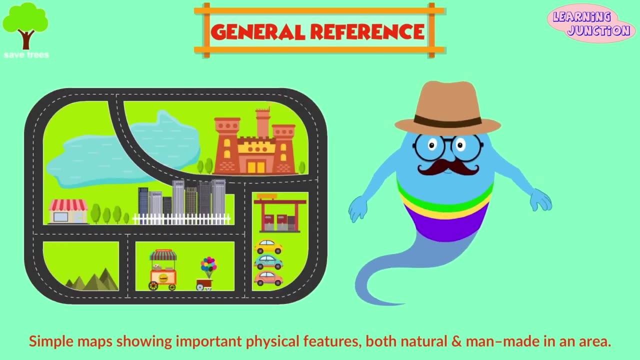 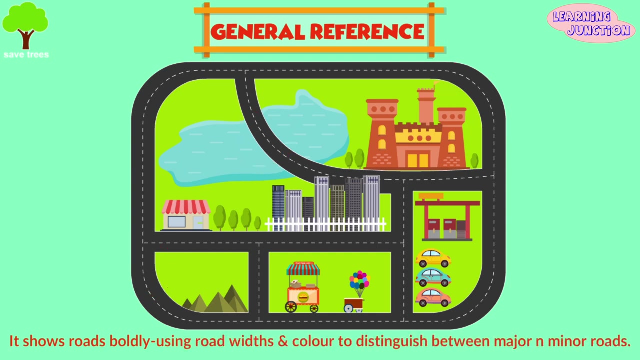 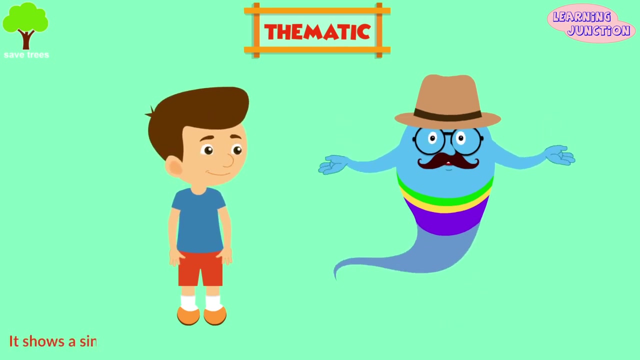 General Reference Map. These are simple maps showing important physical features, both natural and man-made. For example, see this road map. It shows the roads boldly and using road widths and colors to distinguish between major and minor roads. Thematic: A thematic map shows a single attribute. 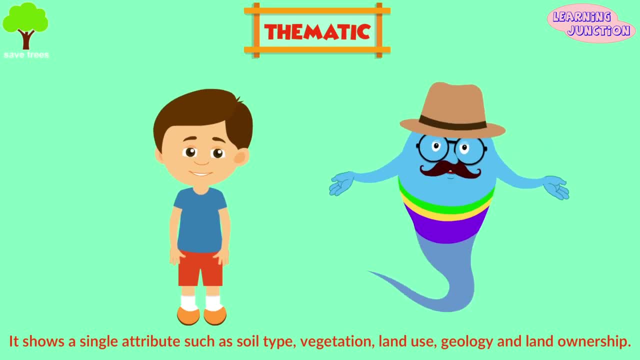 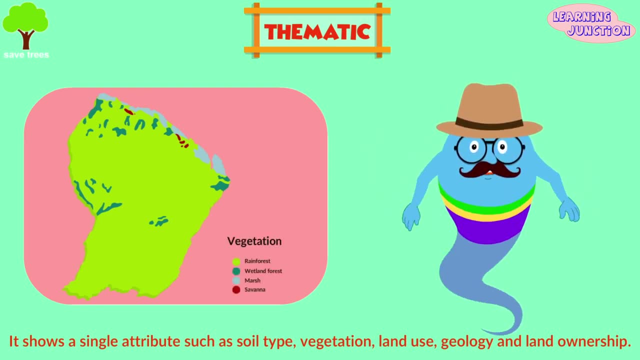 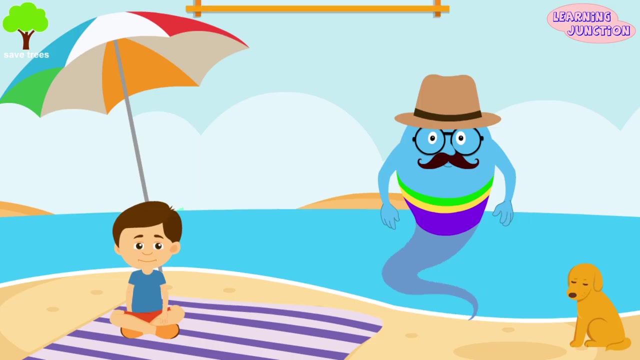 such as soil type, vegetation, land use, geology and land ownership. For example, this French Guiana map shows the vegetation areas, The rainforest areas, Westland Forest, Marsh and Savannah Navigation Charts, or Nautical Charts. It is a map that characterizes the 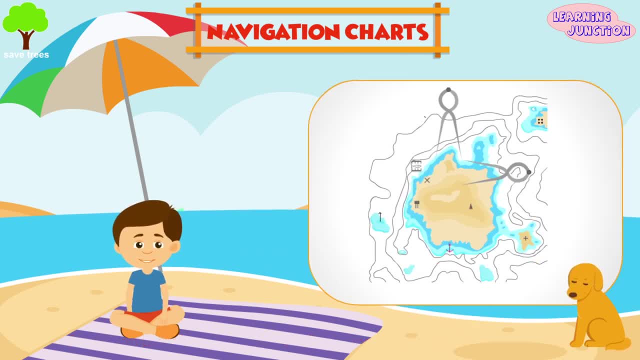 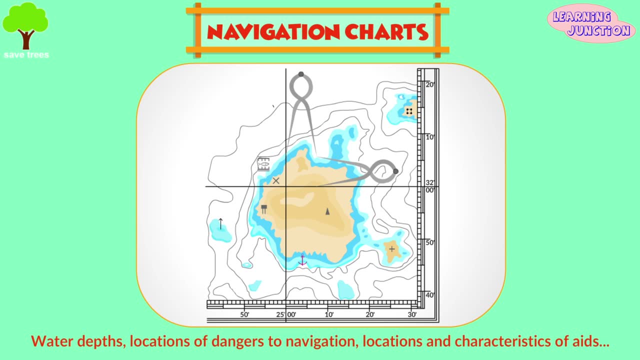 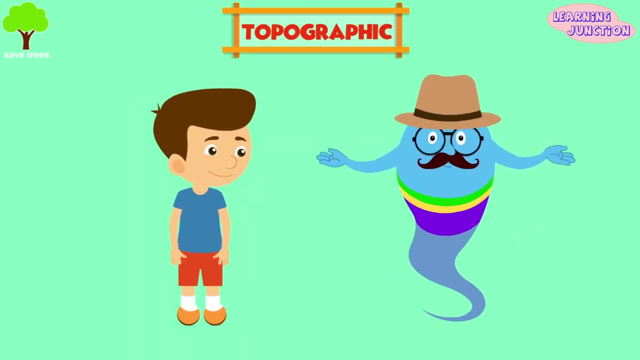 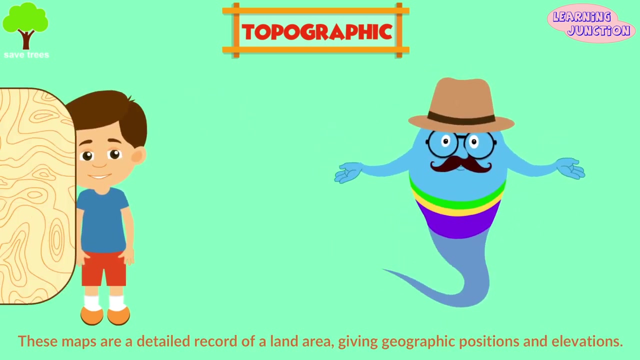 configuration of the shoreline and seafloor. It gives important information about water depths, locations of dangers to navigation, locations and characteristics of aids to navigation, and many other features. Topographic Maps: These maps are a detailed record of a land area, giving geographic position and elevations.